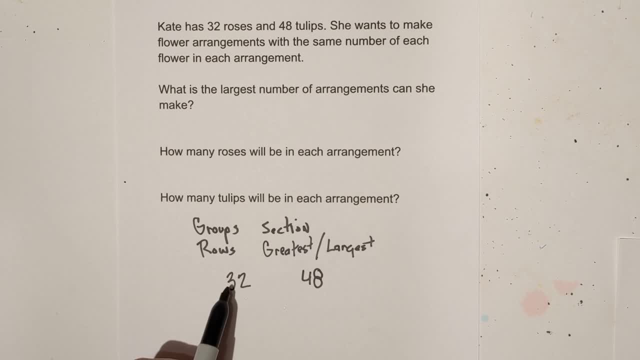 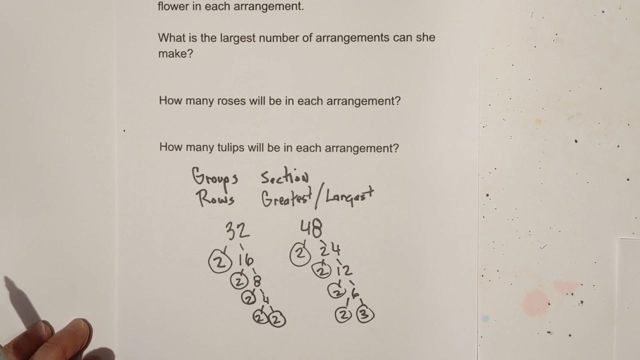 so it's going to be equal to 32 and 48.. equal to or less than 32, or equal to or less than one of these two numbers. so let's get started. I know that. okay, to save a little bit of time, I went ahead and drew out the factor tree for each. 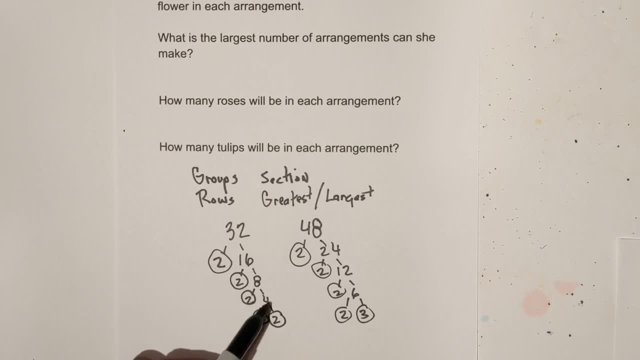 one 32, 2 times 16, then 2 times 8, 2 times 4, 2 times 2.. okay, if you need to know how to do a factor tree, I'll leave a link for a video on how to do this. now here's something that is really really. 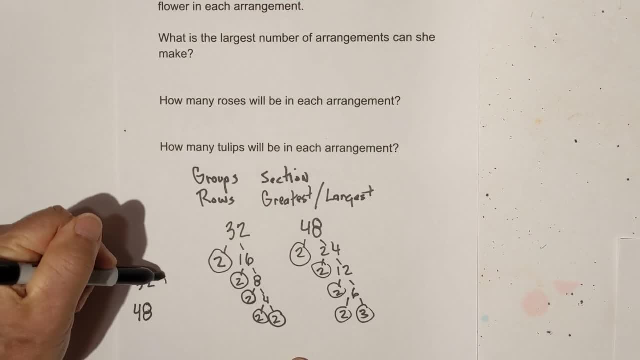 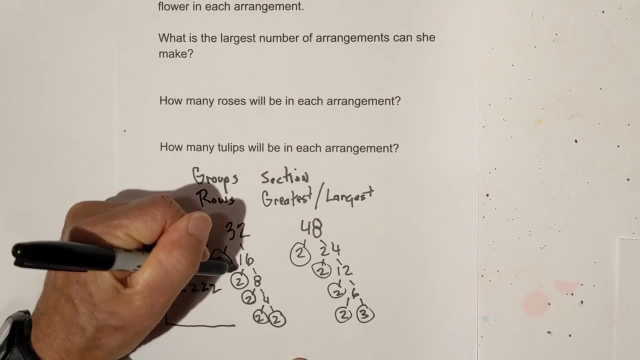 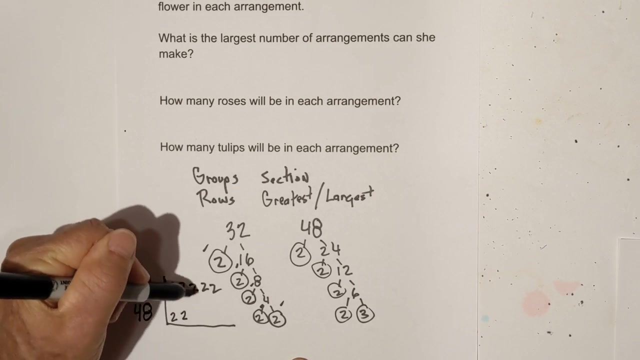 helpful. what I do after this is I place them in a small chart, okay, so I'm going to write 2, 2, 2, 2 and 2- okay, and then I'll do the same for 48. it's got a 2, then a 2, a 2 and a 2- okay, and then a 3 and notice. 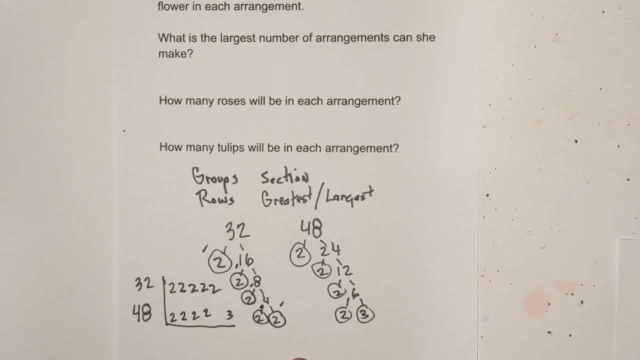 I'm going to skip over this, because it's not a 2.. and the rule for the greatest common factor is: you have to get a number and you have to get an variable in order to know that you have a 2, as well as you have to write the number and you can take the number at any given moment. let's say: 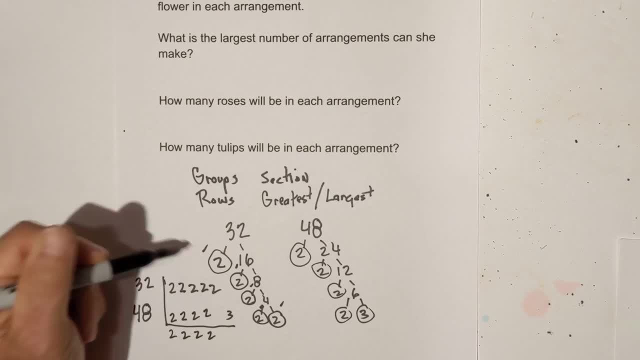 where we have the 2 on the chart and you have the number 1, the number 2 here and then 6 on the chart and you multiply that by the number 2, you get the 16. that's a year thing, and in this case we 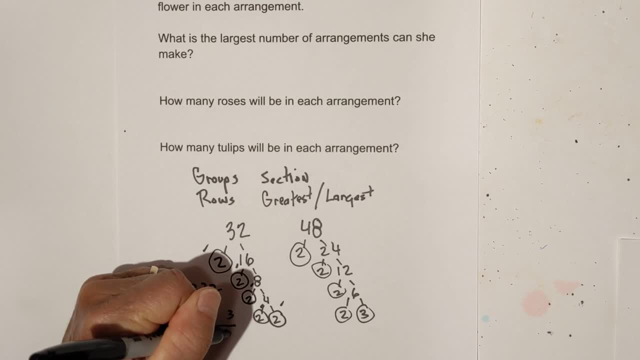 have two numbers when you need to have 2 numbers in each column in order to bring it down. so there's a 2 here and a 2 here, and a 2 there and a 2 there. I do not bring down this 2 because there's not another number there, and the same with the 3, and then you just multiply these together and that will give you your greatest common factor, which is 4 and 8. looks like 16.. let me double check my math and yes, 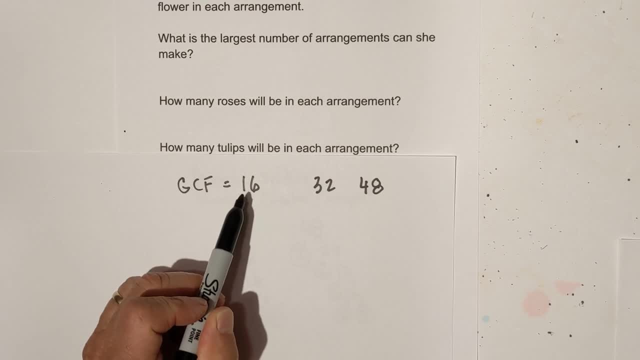 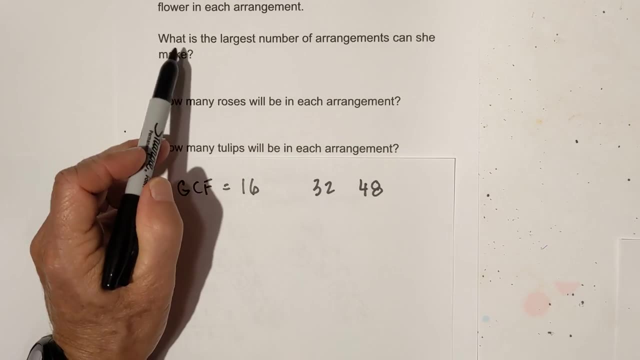 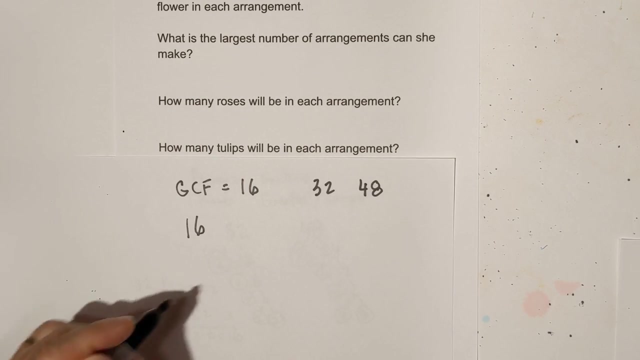 we got eight in there, math, and yes, that is correct. so now i know that the greatest common factor for 32 and 48 is 16. so let's answer these questions: what is the largest number of arrangements she can make? well, that will be 16. how many roses? well, they have 32 roses. i'll put an r there and a t here, and so you. 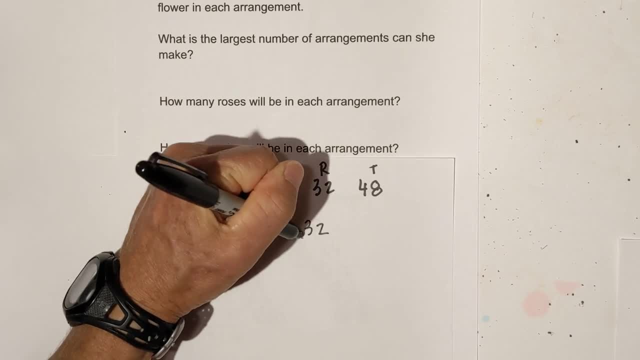 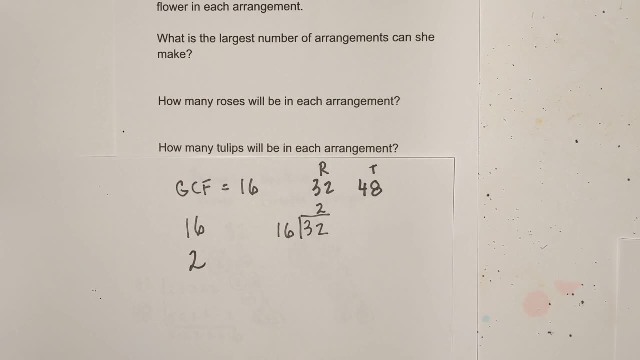 take 32 divided by 16, and that is 2, so you can make you place two roses in each one, and then for 48, uh, how many tulips you take? excuse me, i got ahead of myself- how many tulips will be in each arrangement, and that is 48. so 16 divided by 48 is 3, so you'll have three tulips. so in summary, 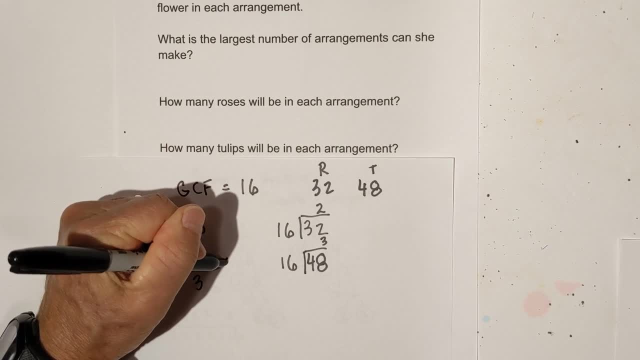 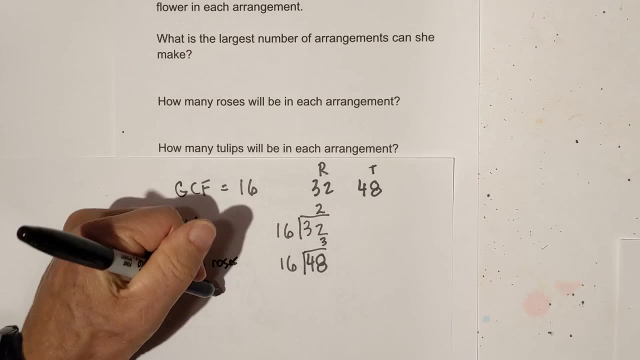 you'll have 16 groups. you'll have two roses and the way i got that was: i took the number of roses and divided by the greatest common factor and then you'll have three tulips in each arrangement. the way i got that, there's 48 tulips and i divided it by the greatest common factor of 16, so that is three. 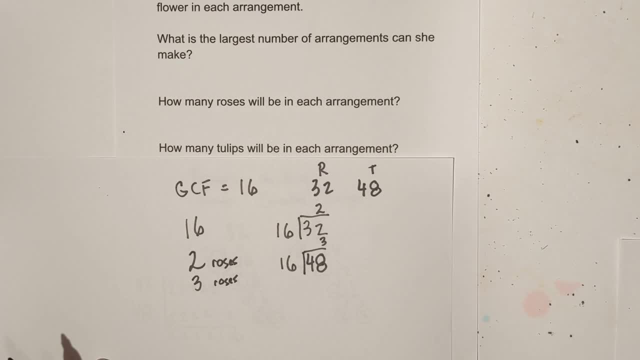 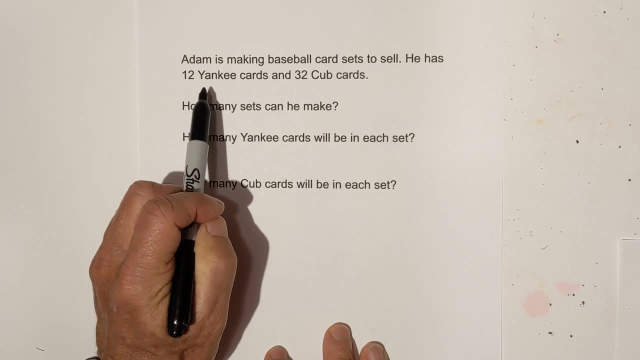 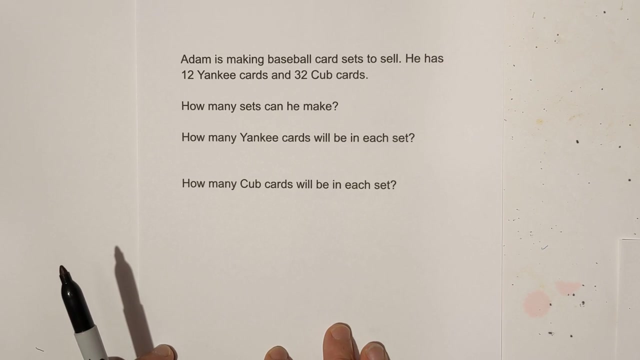 so there's problem number one. let's work another example. okay, example number two: adam is making baseball card sets to sell you. he has 12 yankee cards and 32 cub cards. how many sets can he make? how many yankee cards will be in each and how many cub cards will be in each? okay, first again, greatest common factor: it doesn't act. 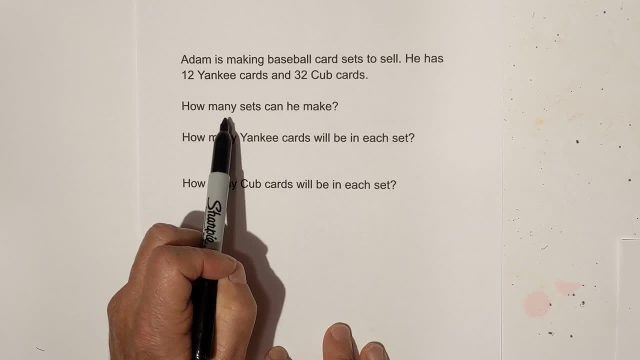 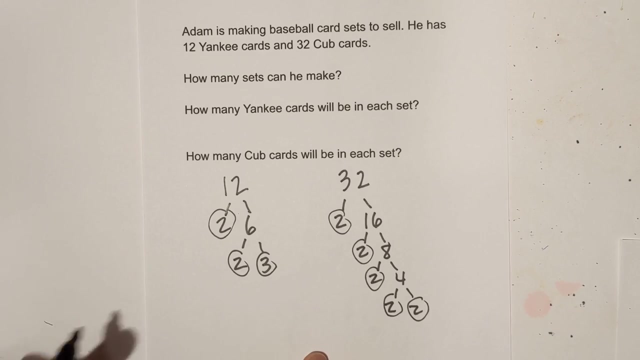 ask for the greatest or largest, but it's asking for sets. remember, groups, rows, sections, sets are all clues that it's a greatest common factor problem. so let's first find the common greatest common factor of 12 and 32. フstop again, i'm going to use a factor tree and i will speed things up. 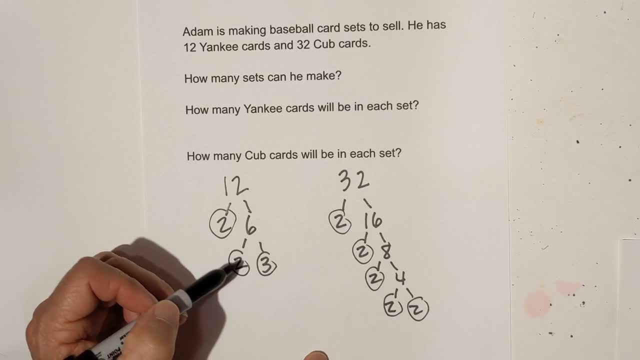 so hang on, okay. so i went ahead and created a factor tree for each one: 12 two times 6 is 12, 2 times 3 is 6. i circle the prime numbers: 32ix, littlepath- pretty good- 36, 37, so manyyle. 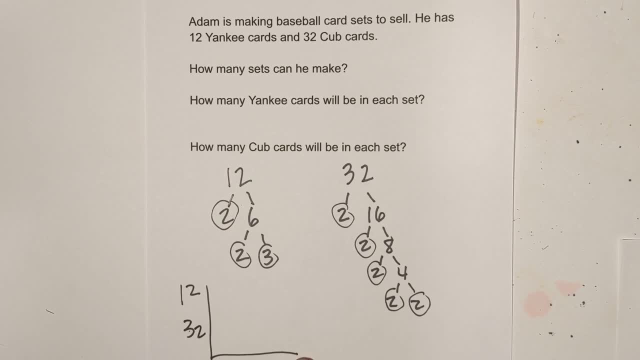 36, 37, 28, 28, 17, 40, 2000, 12, 54, common factor. i just think it's the easiest for myself, so i'm going to write the numbers. okay, i'm going to write the two. the two i'm going to skip here because i don't have another two here. 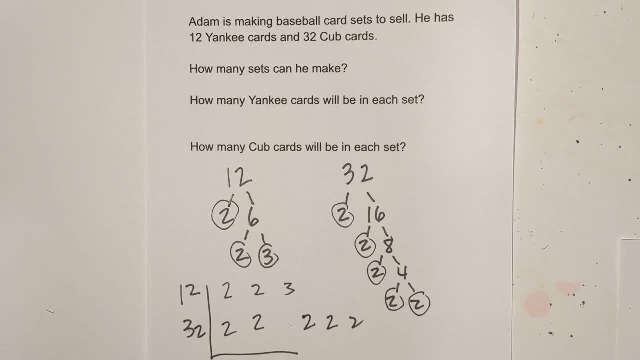 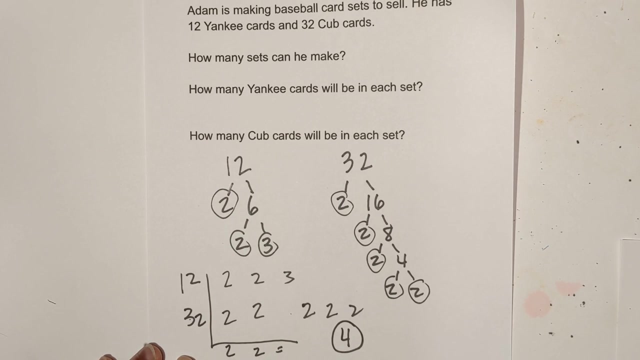 two and two. remember the rule is if you, you have to have two in the column. so i have two and two, which is equal to four. so the greatest common factor- it's barely on there, isn't it? greatest common factor of 12 and 32 is four. now let's see if we can't solve the problem. 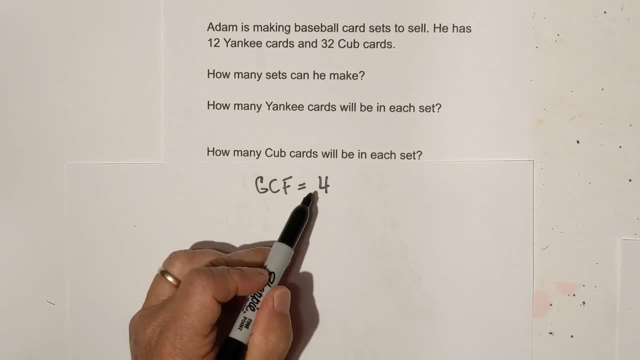 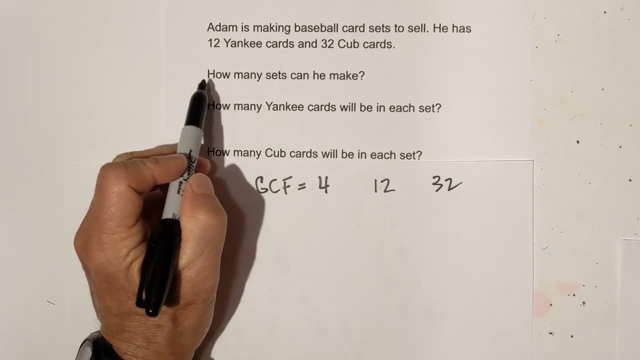 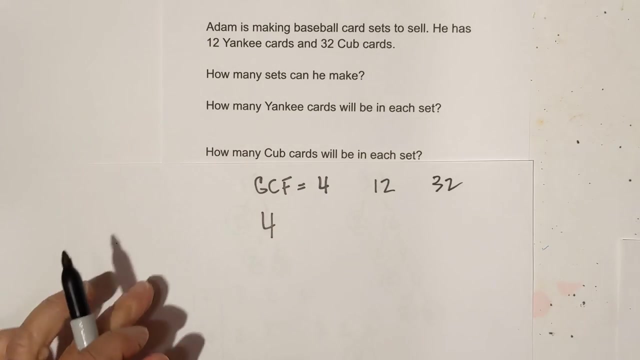 okay. so now we know that we have the greatest common factor of four. we have 12 yankee cards and we have 32 cub cards. so how many sets can we make? well, we know that we can make four sets, because that's the greatest common factor. now, how many will be yankee cards? you? 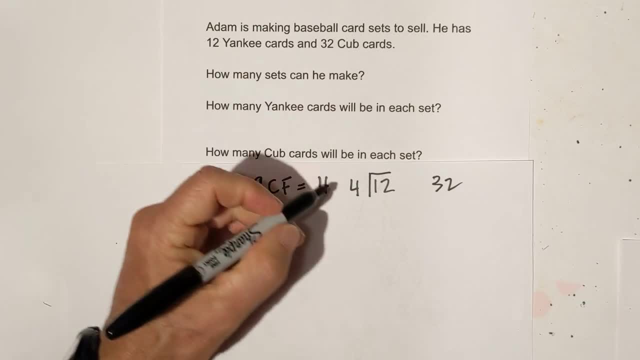 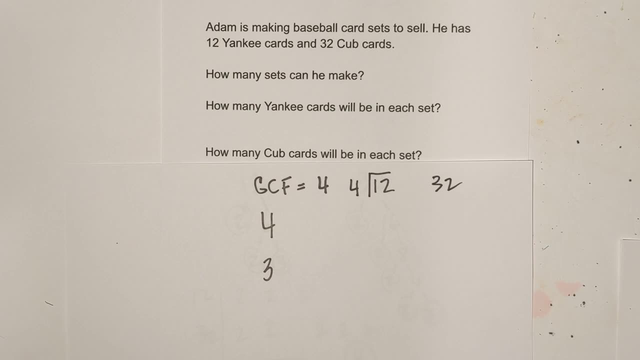 basically just take the number of yankee cards and divide it by four, which is four goes into 12 three times. so you're going to have three yankee cards in there. and now for cub cards you take 32 again. divide it by the greatest common factor and four goes into 32 eight times. 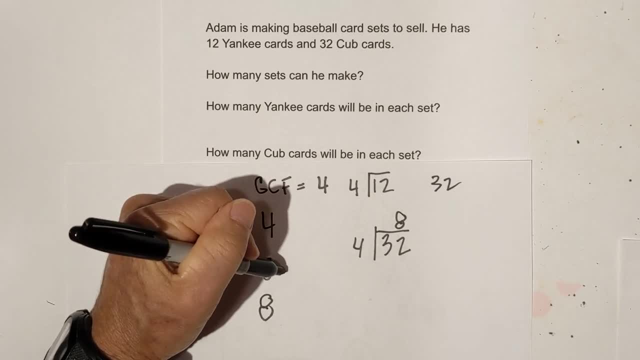 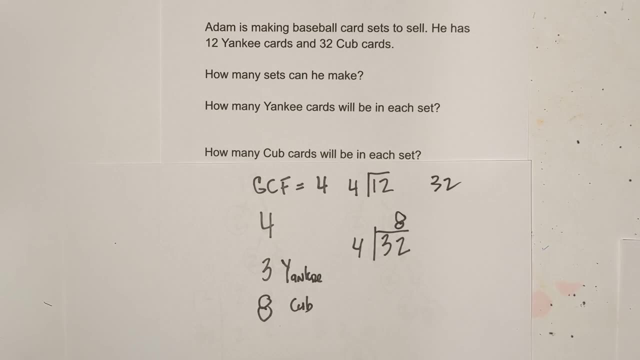 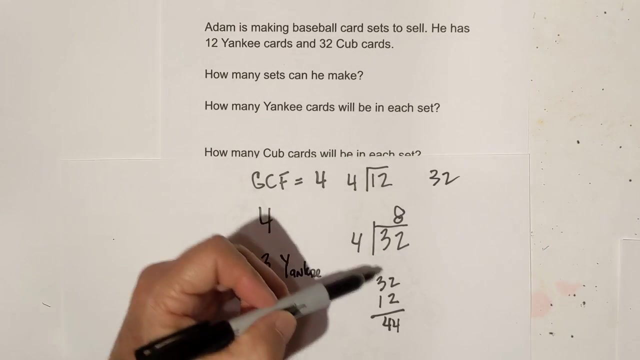 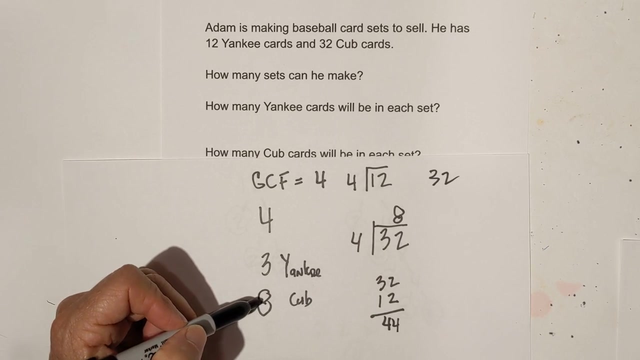 okay, and so you will have three yankee cards and 32 cub cards. so now, if you would like to check your work, notice that you have 12 yankee cards, 32 cub cards for a total of 44. you're going to have eight cub cards, three- excuse me, three- yankee.